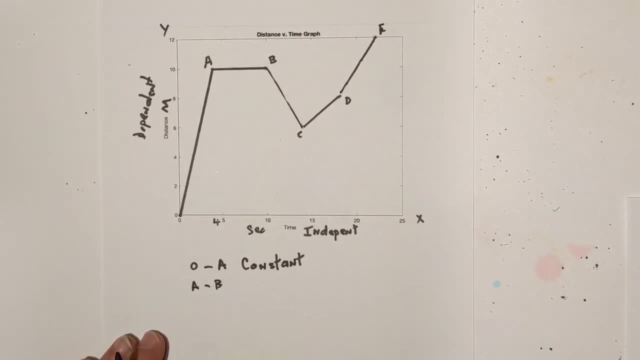 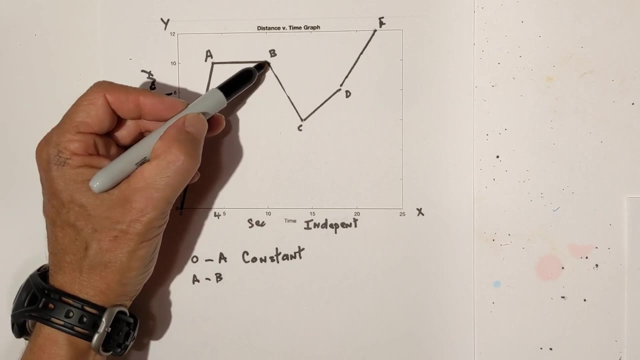 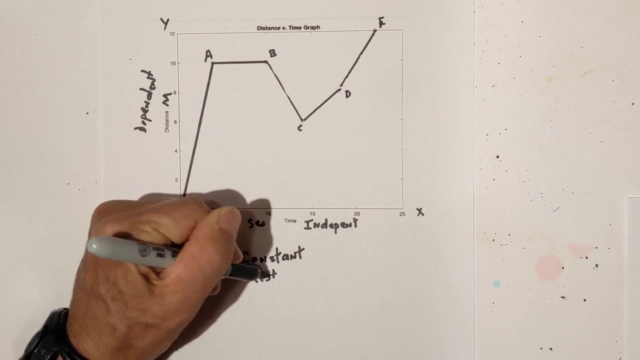 from a to b. Am I still on? Yes, From a to b. it's going from ten to ten in roughly from six seconds to ten seconds. So what you have is it's going to be at rest because it's not going. 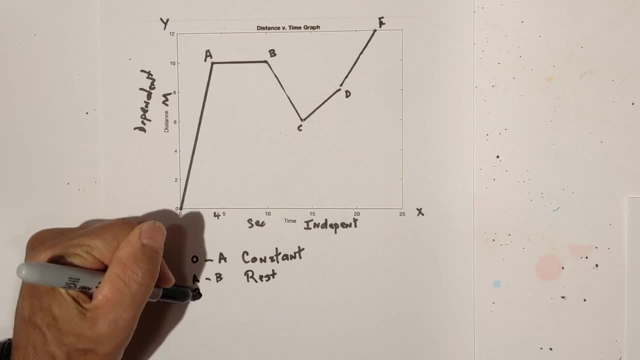 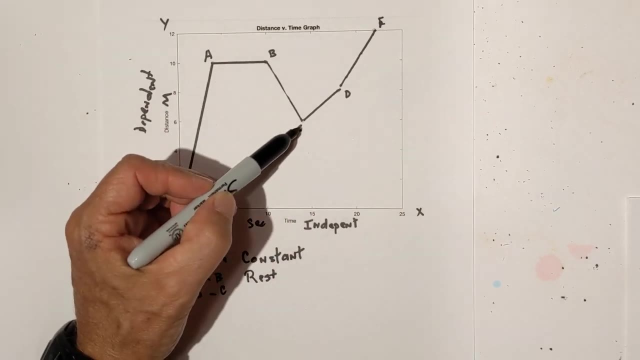 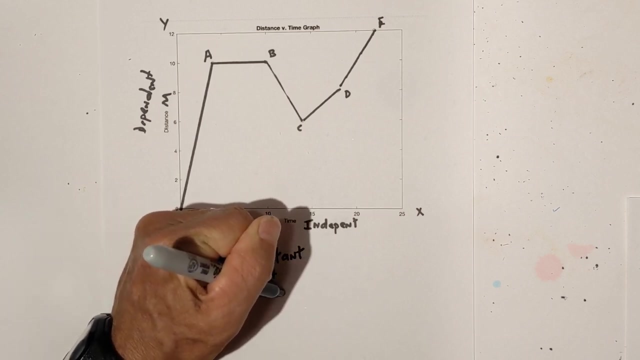 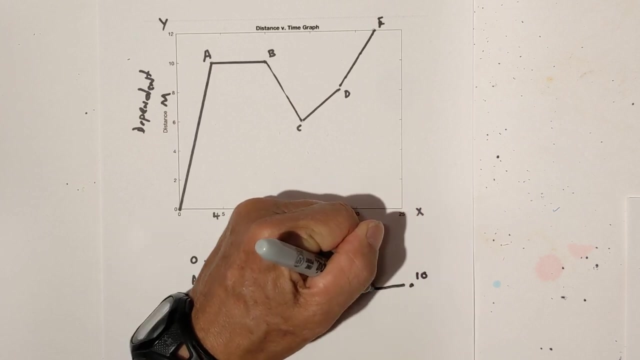 anywhere. Now let's look at from b to c. From b to c, it's going from ten meters now down to six meters. So it is actually the movement is constant, but it's going in reverse. Okay, Because it wants. it was at ten meters, Okay, And now it's back here. 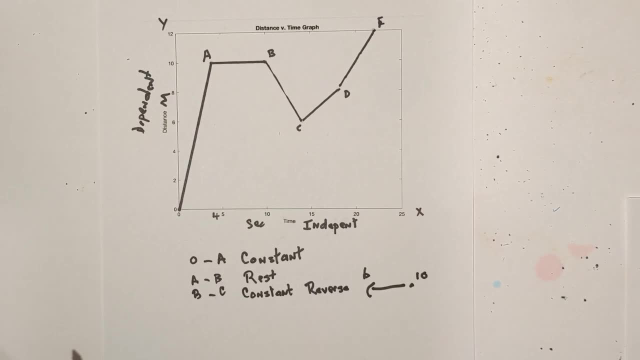 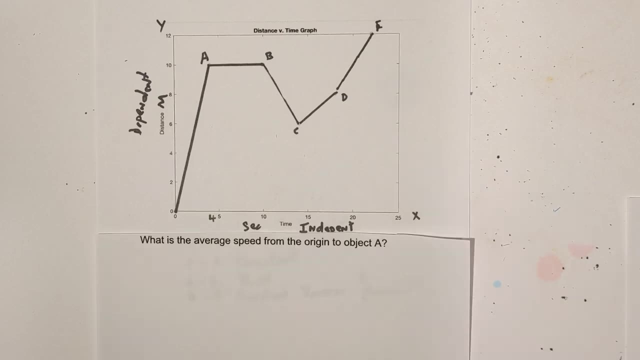 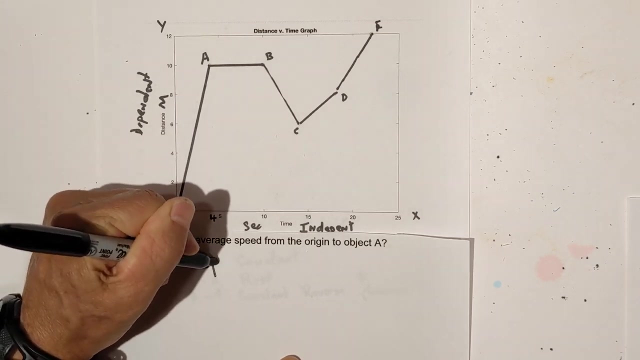 at six, And that's what it looks like. It's going down, so it is in reverse. Now let's begin to calculate some speed, average speed problems. Okay, Here's how we calculate average speed. Average speed is basically the slope, And you know. 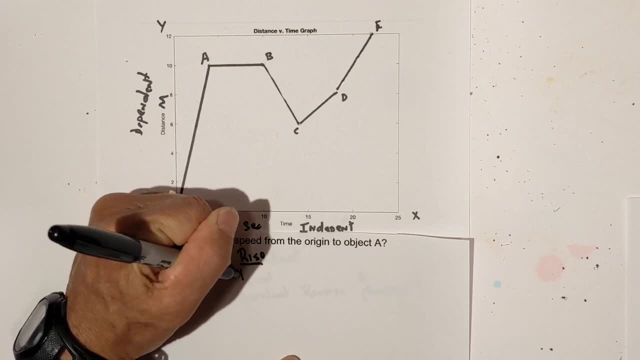 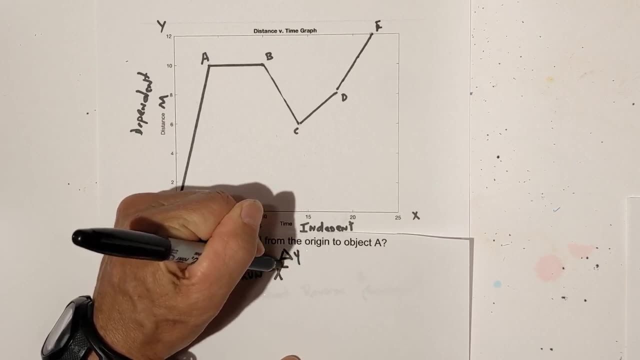 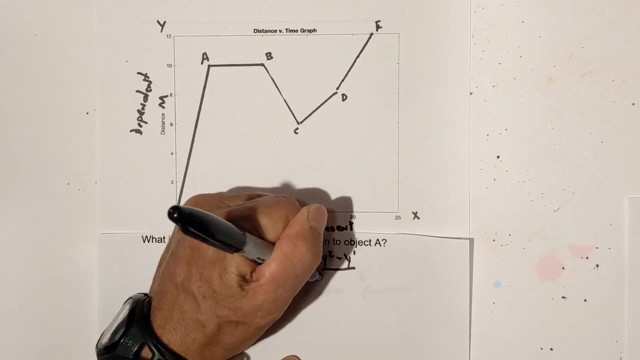 the slope is defined as rise over the run or change in y over change. Oops, My pyramid's upside down. Change in x. Okay, And you can define this as y two minus y one over x two minus x one. Okay, That is basically the slope And the 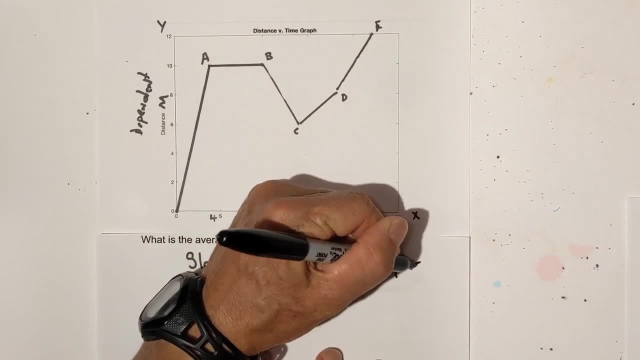 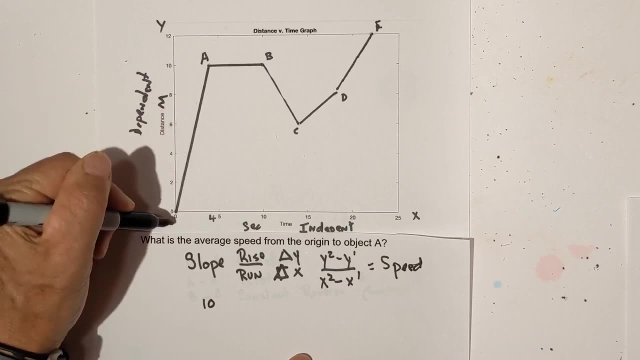 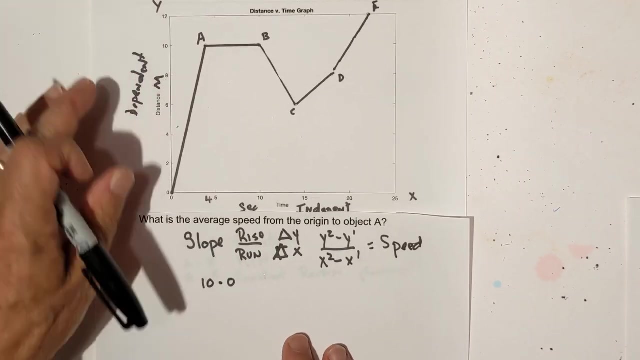 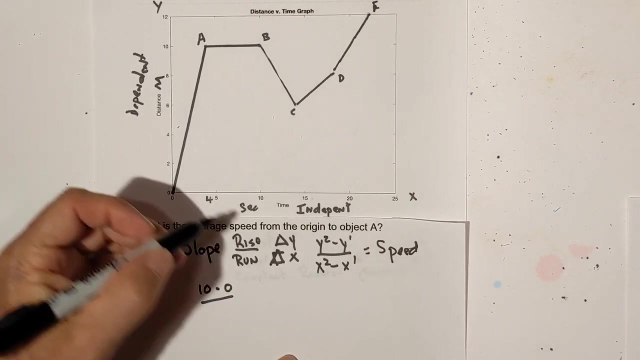 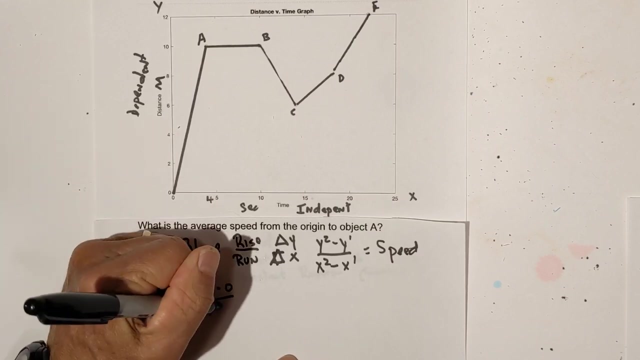 slope is equal to the speed. so let's go ahead and plug some things into the formula: y2 is 10, y1 is 0. okay, make sure i'm still on here. next we have now i got to look at x, x, x2 is 4 and x2 is 4, x1 is 0, so you're going to have 10 divided by 4, which equals 2.5, and now we must. 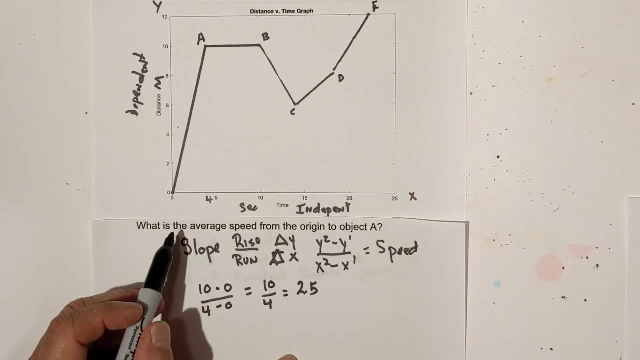 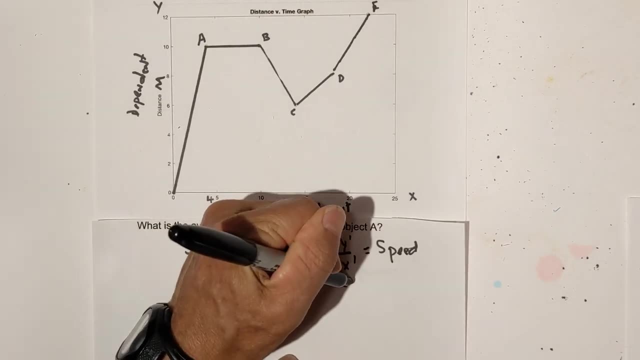 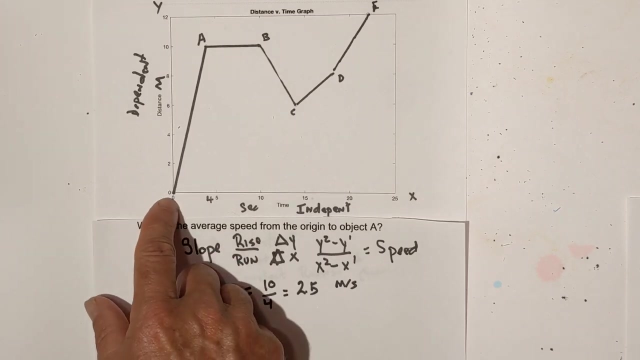 put in our units and the y is meters and the independent is seconds, so it's meters per second. okay, so that would be the, the speed from the origin to a, and i'll put 2.5 meters per second. okay, now let's look at another.